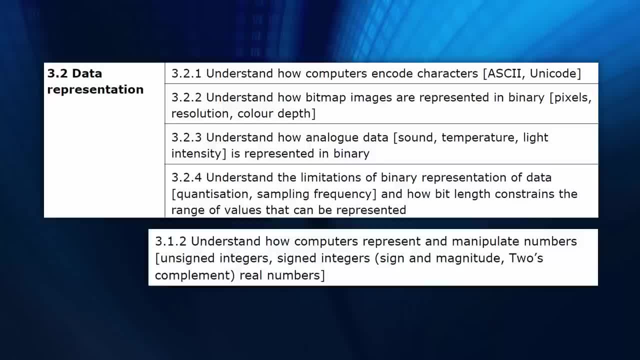 is dealt with in binary. But firstly we need to cover something else, something I missed off the last topic. We need to cover the concept of real numbers and representing them in binary. To be honest, I just completely didn't realise. the way it's formatted confused me a little. 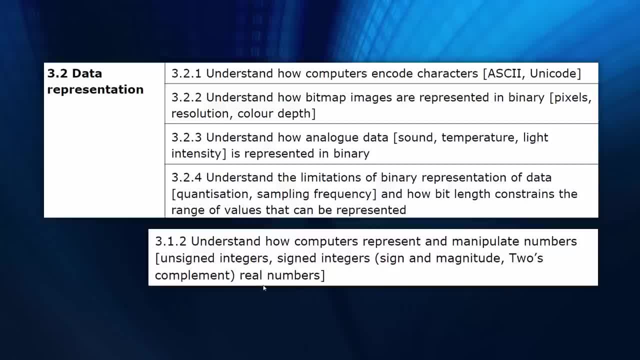 bit because there are some brackets missing, I think. But really I wasn't really looking for it because it's actually introduced in most other courses at A level, so in year 13. Meaning that it seems a bit out of place in a GCSE course. But I looked at a question. 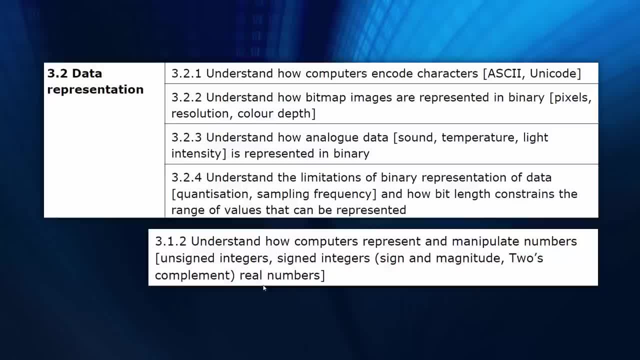 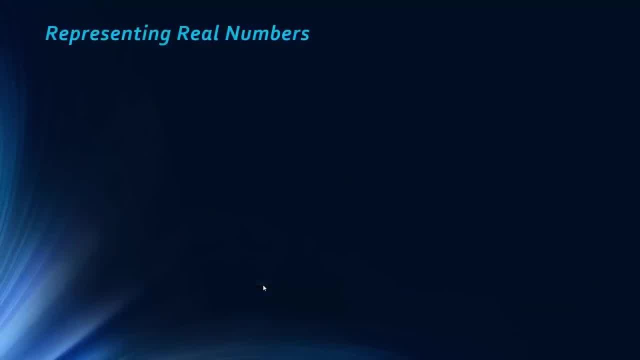 in one of the sample papers on Edexcel's website and there's a question about floating point binaries. So we've got to cover it and, to be honest, it is quite tricky, especially floating point. So we're not going to cover it to the detail that you would at A level, but we're. 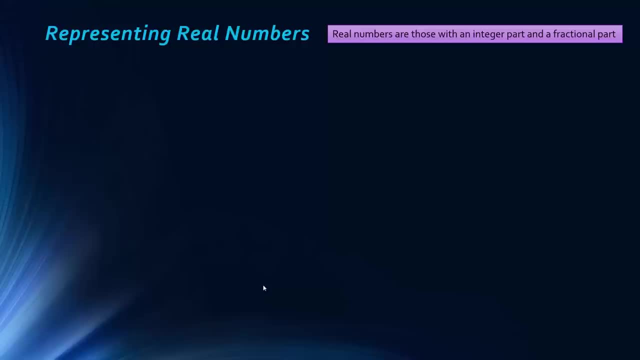 going to cover it, hopefully enough for you to feel comfortable with it, confident enough to talk about it in the exam. so real numbers. firstly, just a recap of the data type video are those with an integer part and a fractional part. so really we're talking about 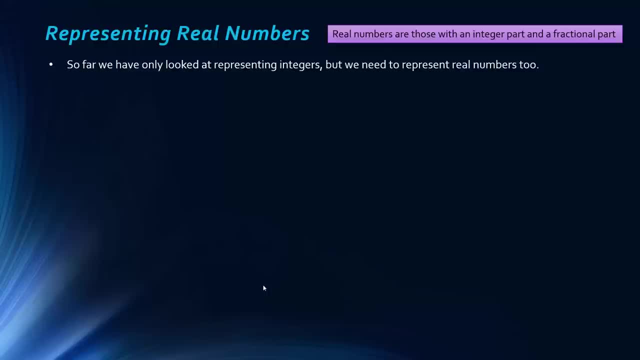 representing fractions here, and so in the previous video we were just talking about integers, but we need to represent fractions too, so the way we can do this is simply by extending the table system. so this is what, for this example, 136.75 looks like in deanery. this is sort of how the 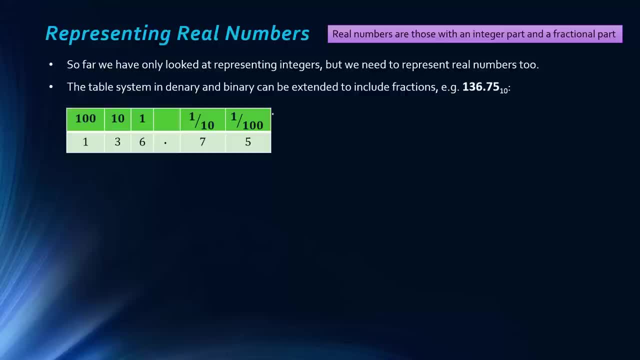 table is broken down. we talked about this a lot in the previous video, so it does actually follow the trend after the decimal point. so we weren't really talking about decimal point, because this was zero. effectively, we're talking about integers, but after decimal point the column headings become 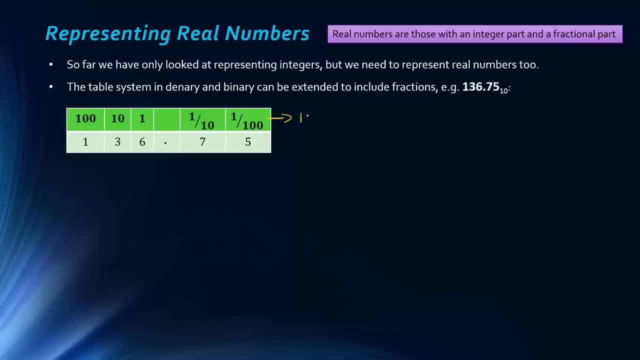 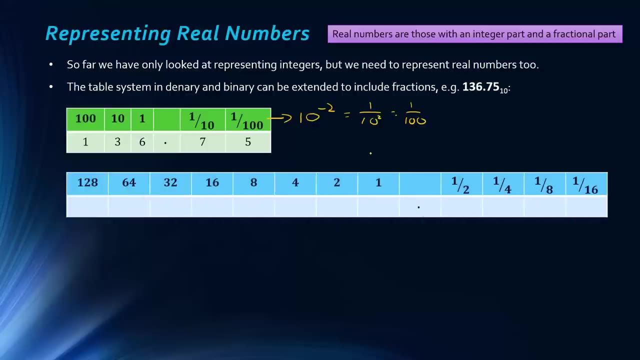 fractions, because what we're doing here we are following the trend by going- this is 10 to the power minus 2, and so this is 1 over 10 squared, which is 100. so that's our column here and you should hope you know this. but what we can do, we can replicate this with binary 2, so this is our. 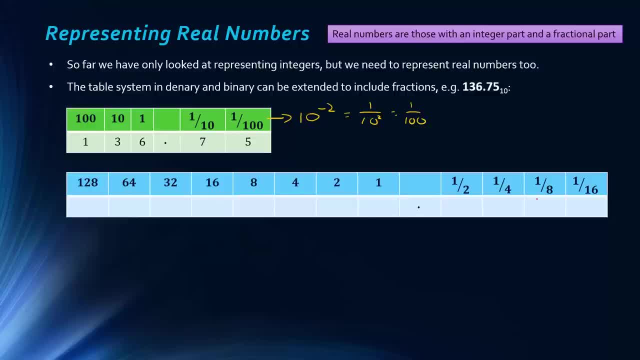 binary table for representing this number now. so if we represent first the integer part, just like we did in the previous video, if I list quickly, this was called the decimal point, so he calls the decimal point. but because we've now looked, we're now looking at binary. 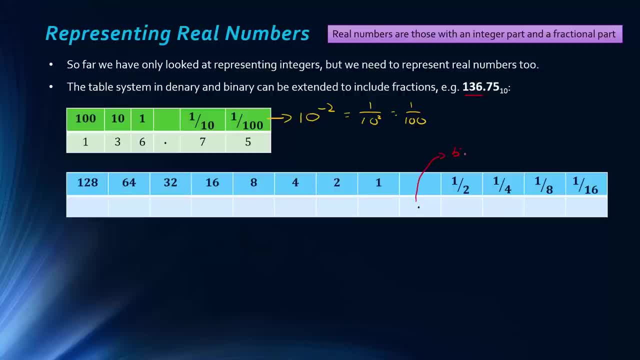 this is now called a binary point also. it's called, so it might be called a radix point, and radix is just another word for base, and so this is also a radix point. it's kind of a general term, but we're now looking at base 2, so we're talking about binary points. this would be talked about as we. 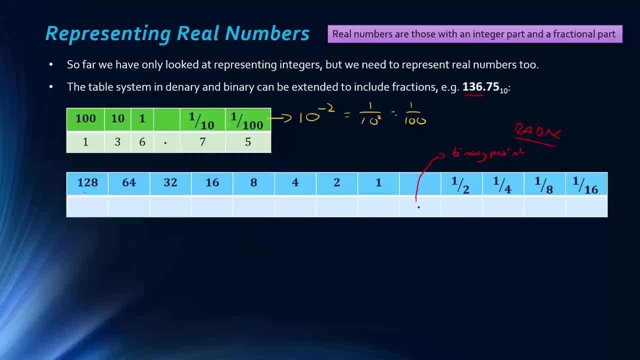 continue this bit, so representing 136 first in our normal bit of the table. so 128 does go in once. so we'll try for me to 8, and so all of these aren't going to go into 8, but 8 is and we've got. 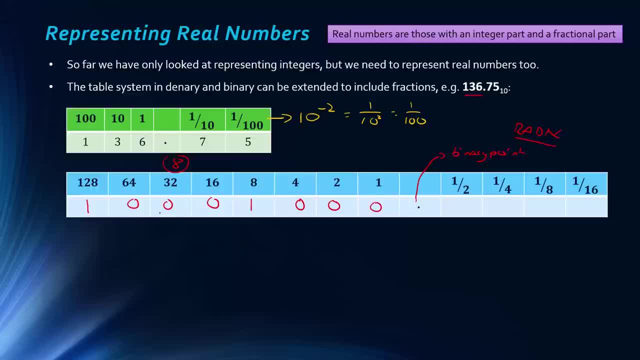 no remainder, so we just write zeros here. so this is our integer part now complete. but after the binary point 0.75 is equal to 0.5 plus 0.25. that's come out not very well. that's a plus 9 times so. 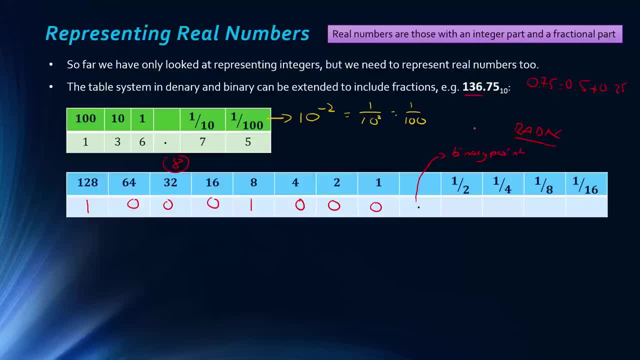 it will be quite. if you do get asked to do this, which I imagine you probably won't in the exam, it'll be quite nice numbers. you can see here we've got a half, because this is going two to the power, and minus one, which is a half, and so on, like this example. so the exponent's getting smaller and 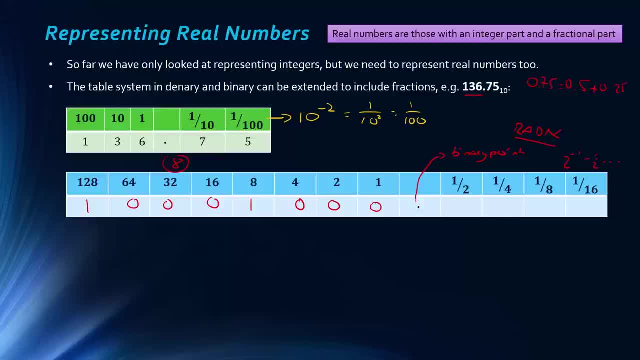 smaller. so we've got one half in this 0.75. as you can see, you've decomposed it and of course we've got a quarter and we've got no eighth, we've got no sixteenths is our binary representation of 136.75, and this is actually called fixed point notation. 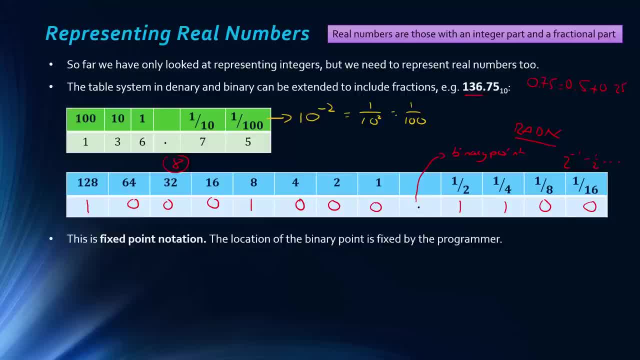 and this binary point is fixed by the programmer. so this binary point doesn't actually move and that might sound kind of obvious, but actually we'll look at a representation in a second called floating point, where it does definitely move. So because there are an infinite number of real numbers, you can keep dividing a number. 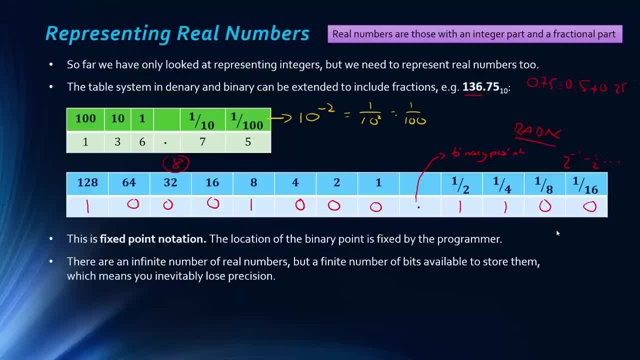 that is infinite. you've only got a set amount of space in a computer, so you are inevitably going to lose precision. The numbers in binary compared to deanery are kind of awkward to deal with conversions so we won't really talk about that. but you are going to lose precision. 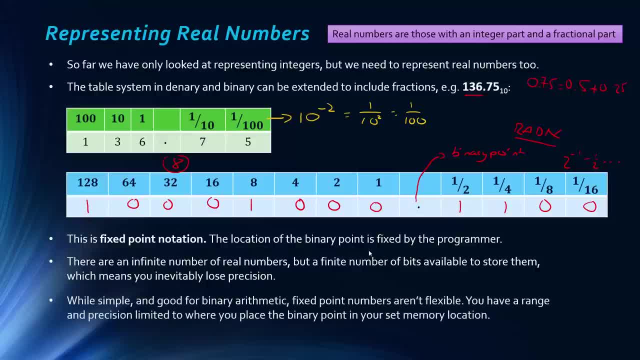 storing real numbers And, as we'll summarise in a couple of minutes, fixed point notation is really good for binary arithmetic and it's also quite simple. this is quite an easy logical process, but they are not flexible because of this binary point being fixed and 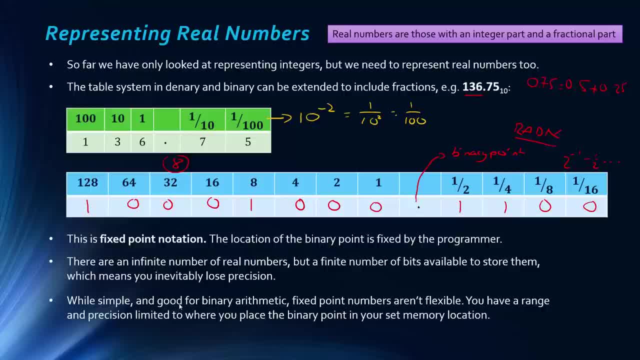 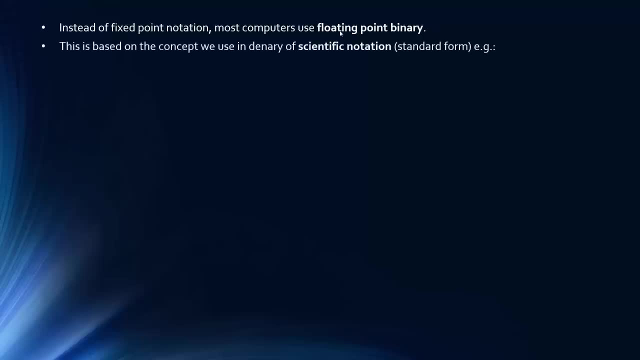 so you can sort of do a trade off: you can increase precision but you have to decrease the range of the available representations. But this can be kind of countered by looking at another representation which is mainly used in computers and that's floating point binary. and this is based on a concept we use in deanery called scientific notation. you 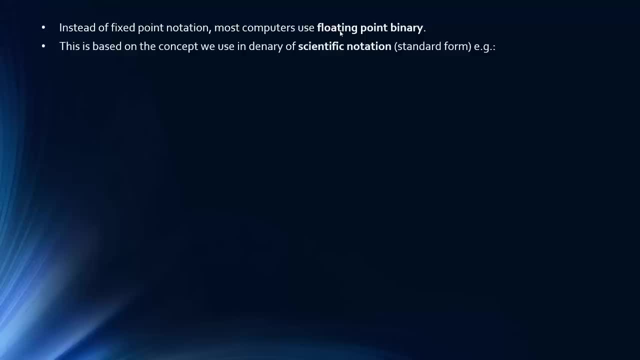 probably know it as standard form. that's what it's called in GCSE maths, I think, and that's what I learned today, And so really it's about collapsing large numbers into this smaller form. So, firstly, million can be written as 3.2 times 10 to the 7, and this small number can be written. 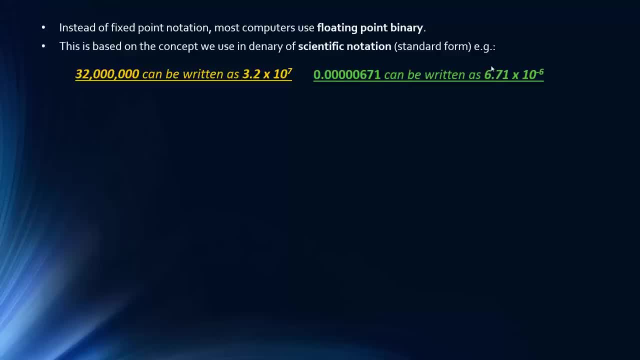 as 6.71 times 10 to the minus 6.. So it's writing it in a slightly easier form and it does help with calculations writing it in this way. And so the way this scientific notation is broken down into is for mantissa, which is 3.2 and 6.71 in this example, multiplied by 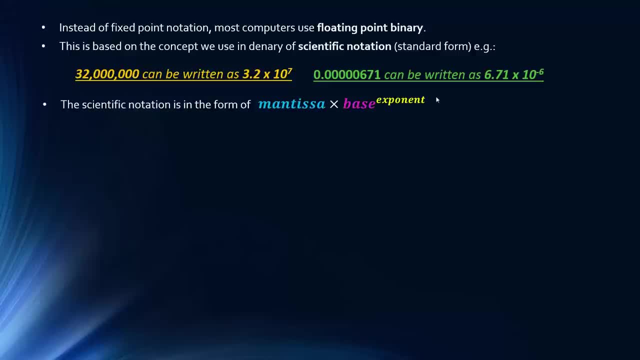 multiplying the base raised to the exponent, and the base is, in deanery, base 10 and in binary it's going to be base 2.. So it's also called the significant and sometimes the coefficient of mantissa, and that's what holds the digits and it has this decimal point embedded within. 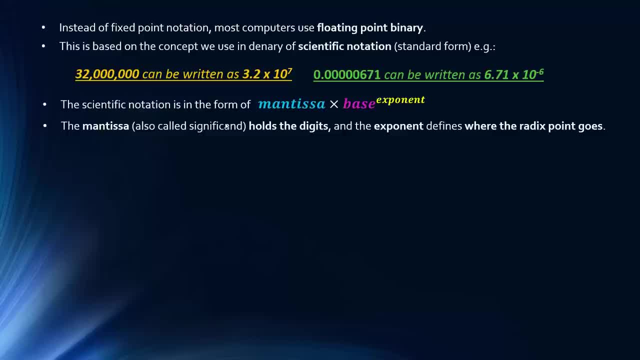 it And the exponent is what defines where the radix point goes. So, as the name quite clearly implies, and as we've just said in the previous slide, the radix point here can move around. It can float. It can move around. It can float. It can float, It can float. 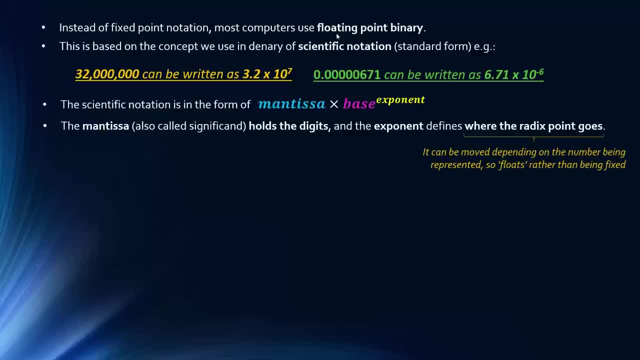 And so, depending on what number you're representing, you might be representing a large number. well then, your radix point can float to a position that can accommodate that, which really adds more flexibility to it compared to fixed point. And so, to replicate this in binary, 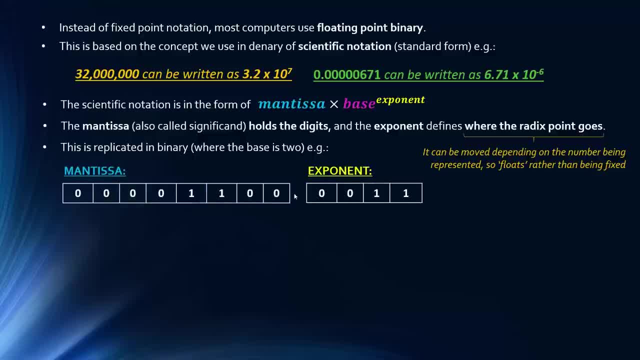 if we have this example. so we've got a mantissa of this binary number and the exponent is this binary number. they'll be written and obviously in a computer they're all going to be conjoined together And you might write it like this, but often they're written separately. 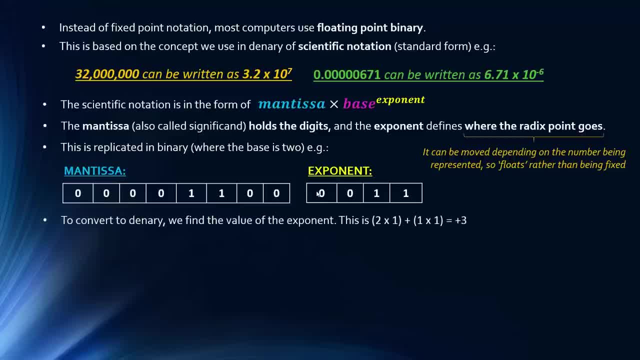 like this, And so the first thing you do if you want to convert from this back to the deanery value- and, by the way, I don't think you'll be asked to do this in the exam, because it is quite difficult, especially when you deal with the fact that actually we're dealing with it in 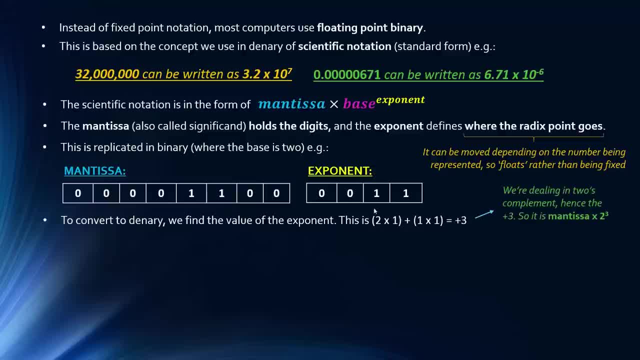 two's complement. You can see we've got a plus three here. So I don't think you'll be asked to do this, but I think you need to watch me do it to understand it. So the first thing we do is we find the value of the exponent. So this is, in binary, just one. one is three. 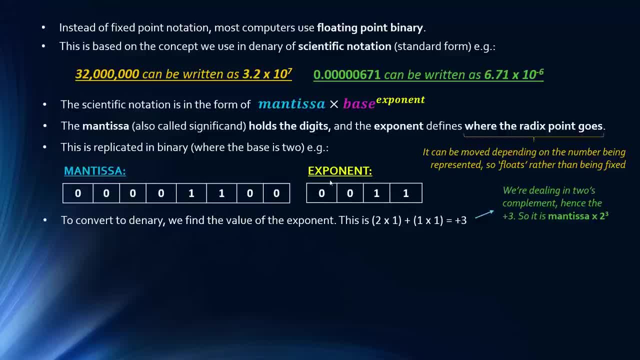 but because we're dealing with two's complement, we're going to find the value of the exponent. This is our most significant bit and this is a zero, so it's positive. so we get plus three. You can have negative exponents, as you can see up here. And so the next step. 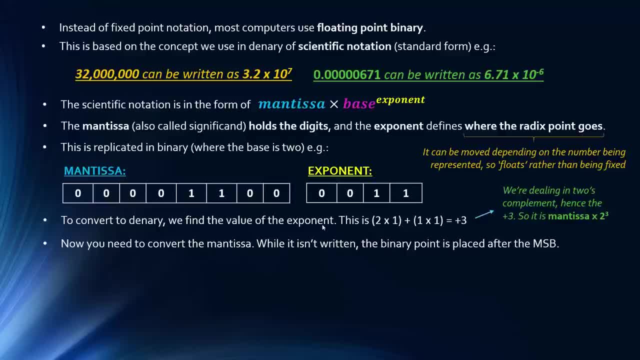 is to convert from mantissa to a deanery number. And while we don't write it, the binary point is placed after the most significant bit. So you can see our binary point appearing here And you can see that in standard form or scientific notation, the decimal point. 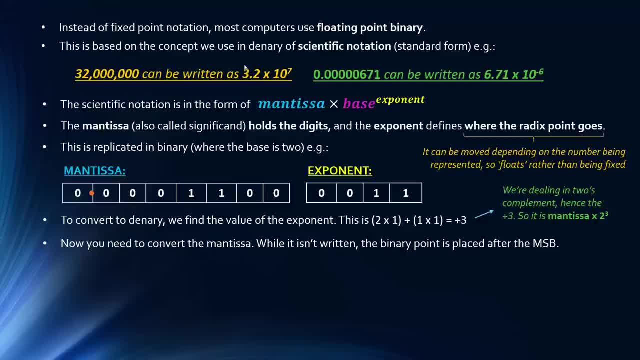 appears after our first digit. It could be a zero, but it doesn't matter. So we're going to write it after our most significant digit or most significant bit, And we don't write it, but it's assumed to be there. And so, from this starting position, the value of the exponent. 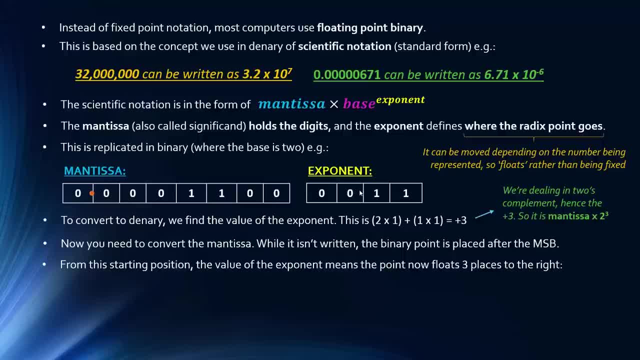 is telling us how far the binary point needs to float, And because we're getting a plus three, it needs to go three places to the right. So we need to add our table. This is our mantissa written in, And so we've got our binary point put in here, And so it's. 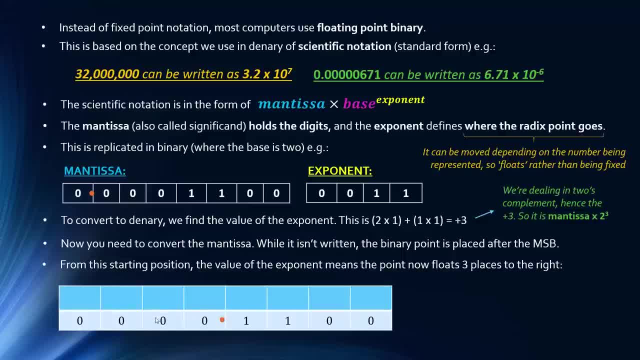 going to float three places to the right, So one, two, three in between the zero and one, And so this means the actual column position or quantities changes, Because I haven't written it in here, but this would be represented as 128,, 64,, 32 and so on. But because of where? 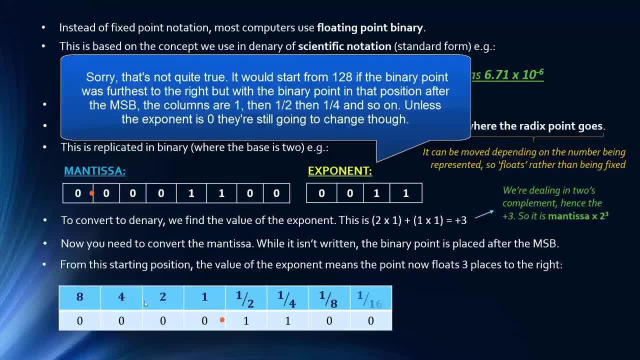 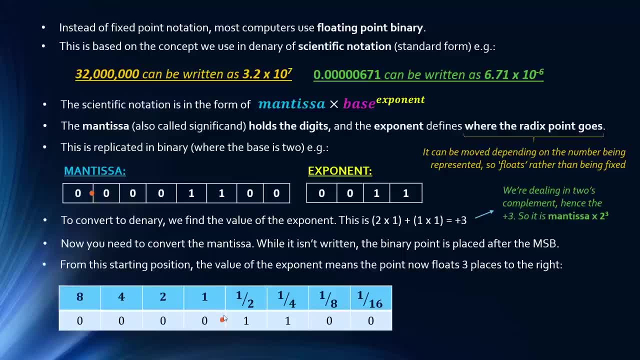 the decimal point is sorry. the binary point is our column headings are changed based on this, So anything to the right of the binary point is going to be correct, It's going to be fractions, And anything to the left is our normal sort of column headings. 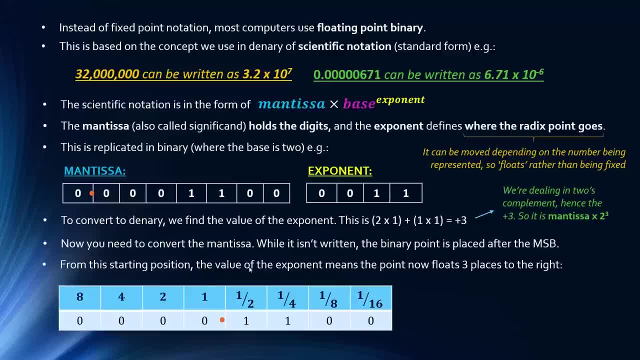 that are increasing times two each time, And so we now just convert it pretty much normally. So this is going to be- we've just got two ones in this representation- So it's just going to be one times a half plus one times a quarter, which is going to be 0.75.. And 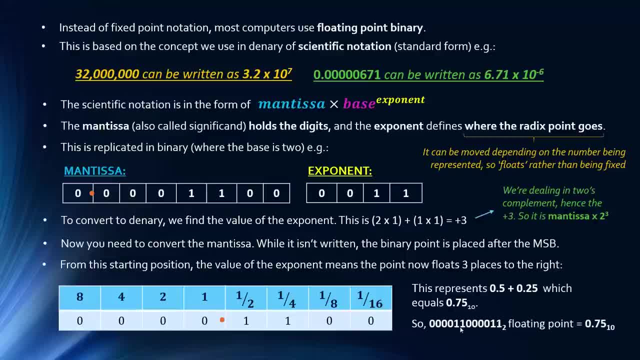 so this. so this is us conjoining it to one binary number. This is just this. plus this together in base two equals our floating point number of 0.75.. So it's quite a difficult process, but there are advantages to doing it like this. 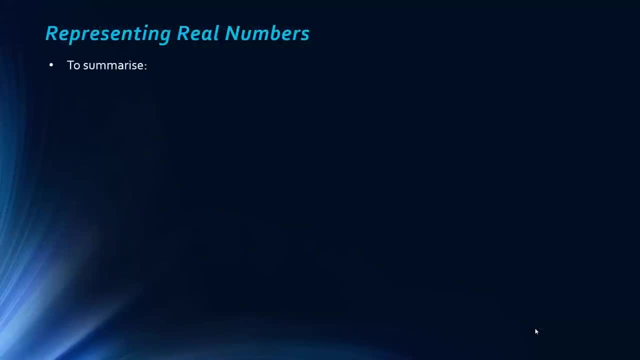 So if we just summarise, this is maybe what you want to try and understand, because you will be asked to do this in the exam, potentially. So the two representations are fixed point and floating point. In fixed point, the binary point cannot move, whereas it can move in. 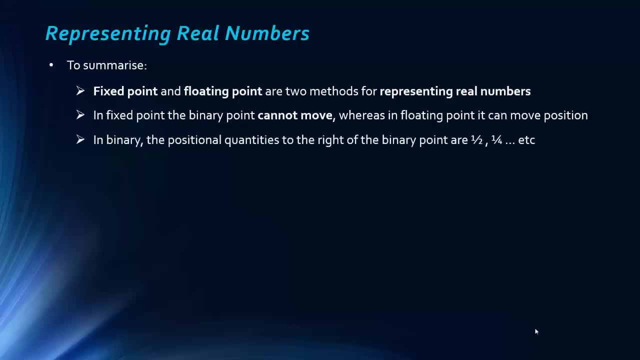 floating point And in binary, when we're talking about representing real numbers, the positional quantities to the right of the binary point go from a half a quarter, an eighth, a sixteenth and so on, And to the left there are numbers. So we're going to go from a half a quarter, an eighth, a sixteenth and so on, And to the left there are. 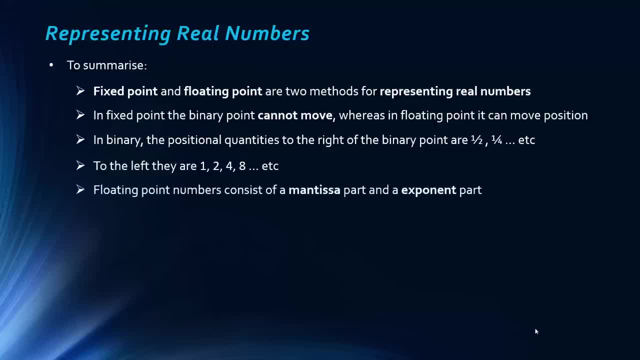 numbers. So we're going to go from a half a quarter, an eighth, a sixteenth and so on. So the main bits to take away from the floating point is that they're broken down into the mantissa part and the exponent part. 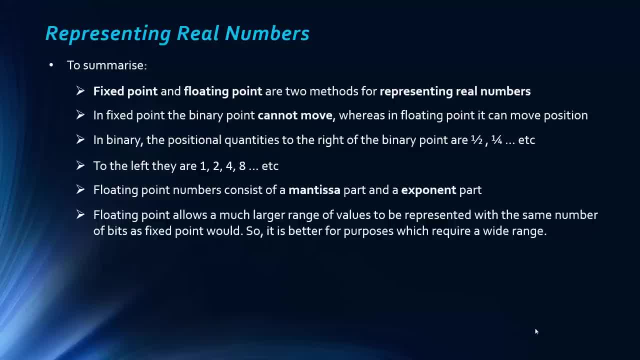 And the advantage of floating point over fixed point is that it allows a much larger range of values to be represented, even though you're using the same number of bits as fixed point would. So it's better for purposes which require a wider range. So you might have a massive number multiplied by a tiny number. 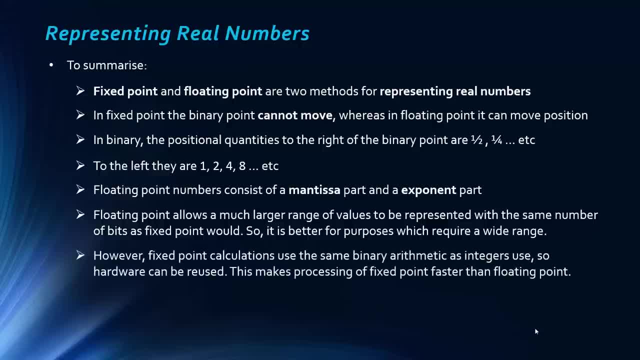 And so slides- And this gives you the flexibility to do that- But fixed point calculations. not only is it actually simpler to do, it uses the same arithmetic as we looked at in the last video, so what integers use, And so the hardware configured for the integer calculations can be used with fixed point too. 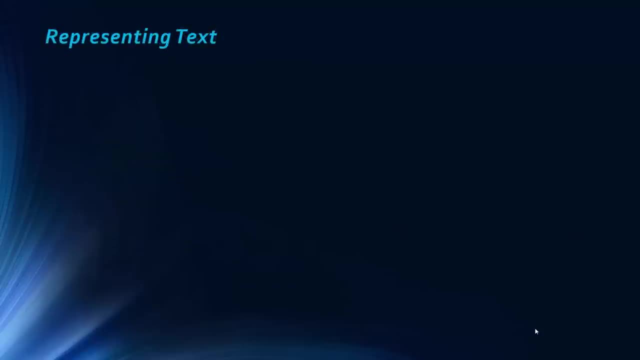 So it does make processing faster, But that's it for this section. This is the previous video, but we're now moving on to actually what this topic is meant to be about, and that's representing text. Okay, so I guess, in comparison at least to what we've just looked at, 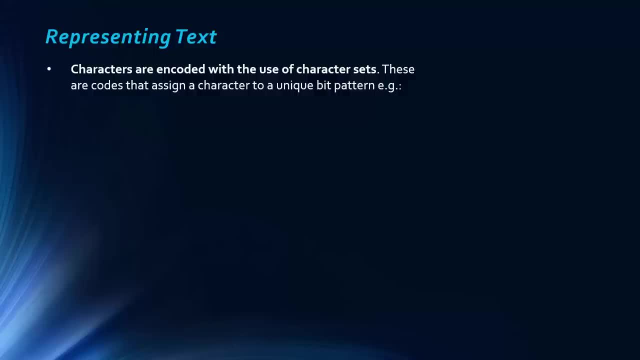 the rest of the video should be relatively easy. So the first thing we need to cover is ASCII and Unicode, And these are examples for two best well-known examples of character sets. And character sets are what are used to encode characters, to represent characters. 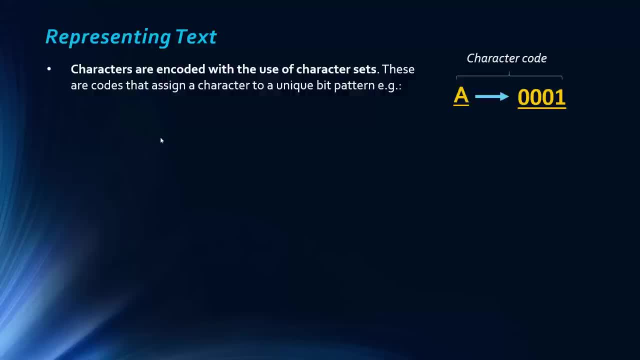 And essentially they're sets of codes that assign a character to a unique bit pattern. So a character code is just a binary representation of a character. So a character is a letter, A letter number or symbol. So in my made-up character set I'm mapping A to 1 in binary. 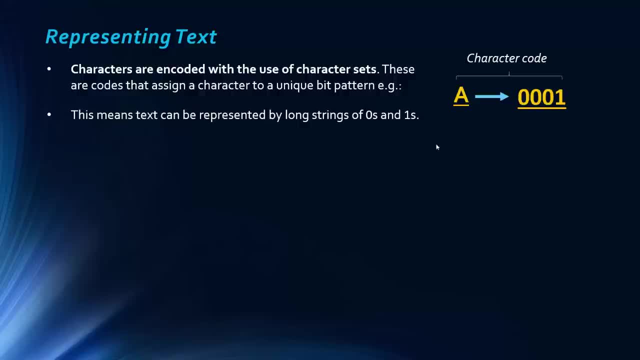 And so the result is: text can be represented by long strings of 0s and 1s, And so a bit of a history lesson here In the early days of computing, so we're talking 1950s, 1960s. 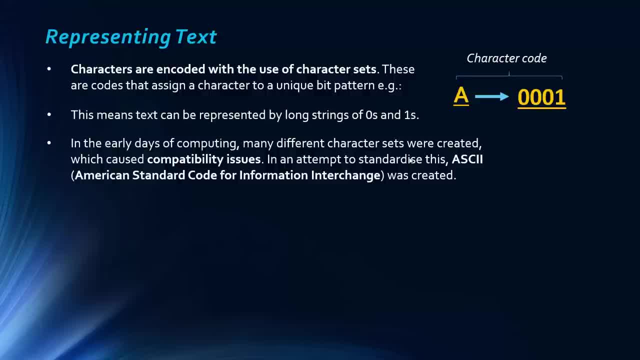 lots of character sets were being created, So different programmers would create their own character sets, And this caused compatibility issues when communication was being introduced to the systems and data. And so, in an attempt to standardise this, something called ASCII was created, And it stands for American Standard Code for Information Interchange. 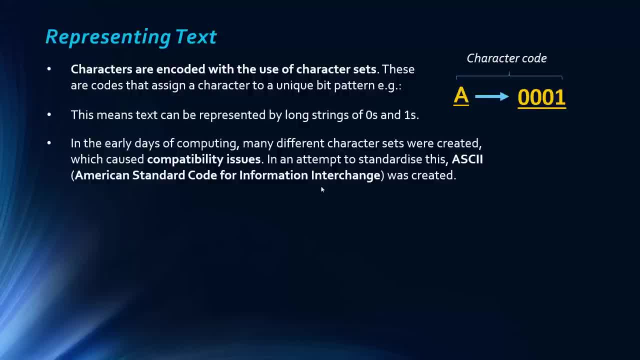 And in the AQA GCSE course there was once an exam question- It was just worth one mark- asking you to write out what it stood for. So if Elic's ever got any ideas, you might want to learn this. So the original ASCII character set. so, like I say, this is talking about 1960s. 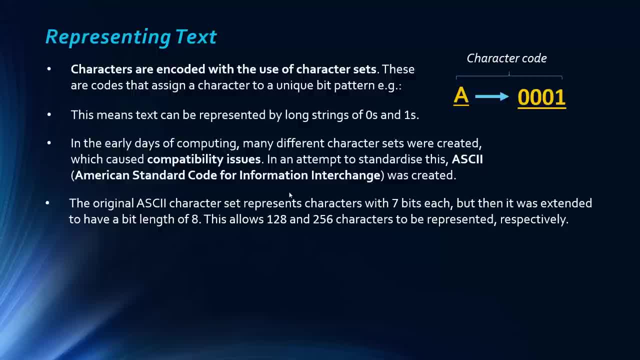 about relatively about that time. It represented characters with seven bits each, But then it was changed to something called extended ASCII to have a bit length of eight, And this allowed 128 and 256 characters to be represented respectively. But even 256 is not sufficient to represent all possible characters in different languages. 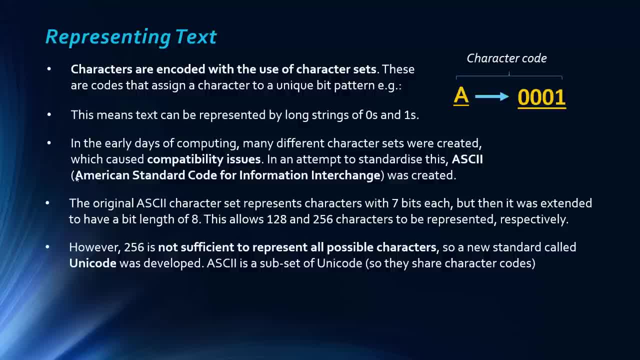 So this was American, so it had the English letters, but it wouldn't have stuff like a pound coin. it would have the dollar, And in different languages which use different symbols, different characters. it's not ideal. And so, when you know, the internet and mass communication was introduced, 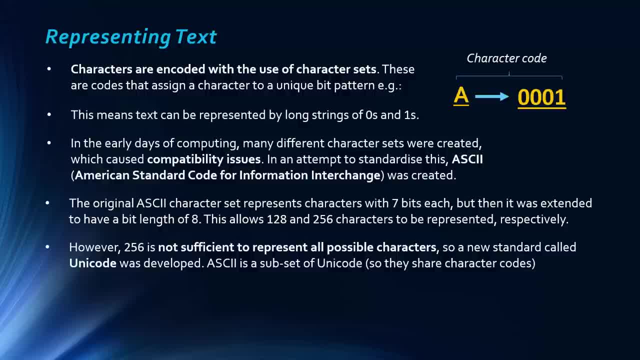 there needed to be a more universal character set, And that is Unicode, And so Unicode was developed to represent more characters And ASCII is a subset of Unicode, so it does include ASCII and they share the same codes And Unicode used. I believe it's changed now. there's been lots of updates for Unicode. 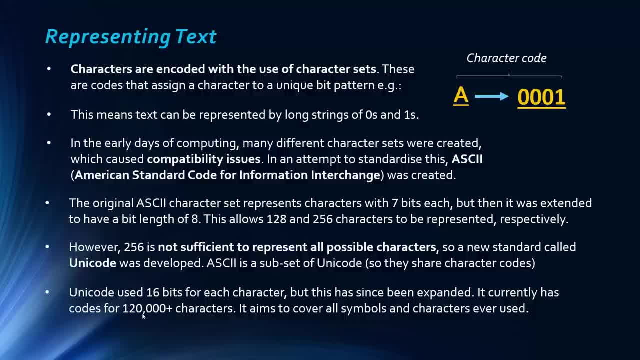 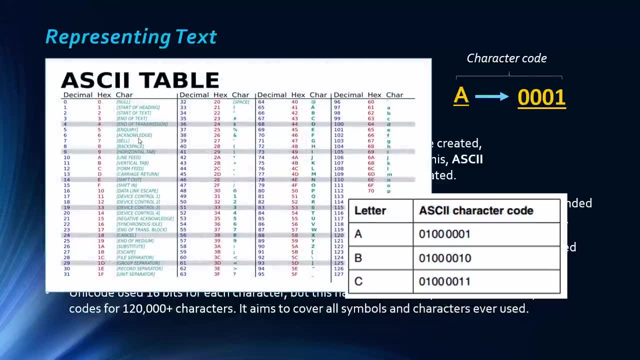 it used 16 bits and 16 bits can represent- or sorry, it can currently code for- more than 120,000 characters, And the whole point of it is to cover all symbols and characters. So this is an excerpt from the ASCII table. 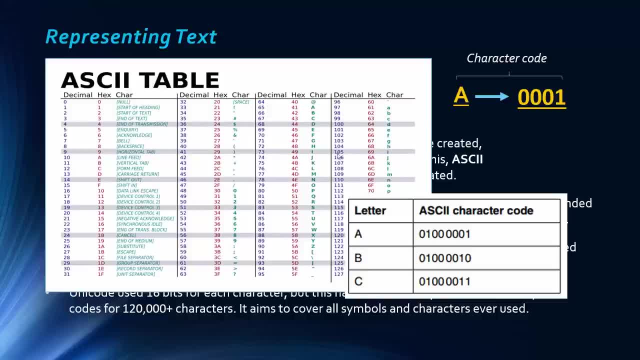 So you can see we've got letters, we've got control symbols And this is what it might be presented in the exam, Just the character code for a certain, for a couple of letters you might have to maybe write out, say BAC. 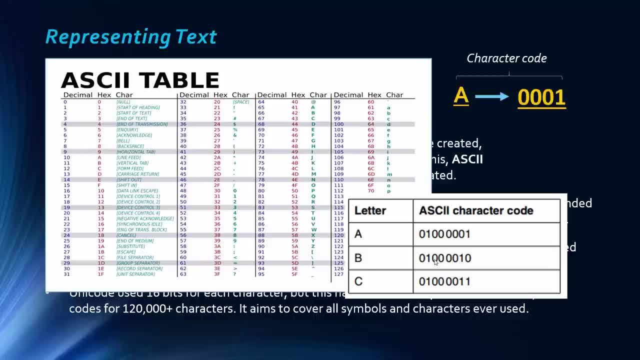 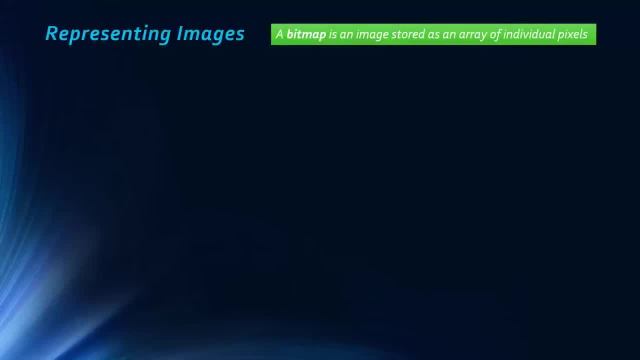 And you literally just write from back to back the whole character code And that's how it will look like, or how it's represented at the base level in a computer. So the next thing we need to look at is this. The next thing we need to look at is representing images in binary. 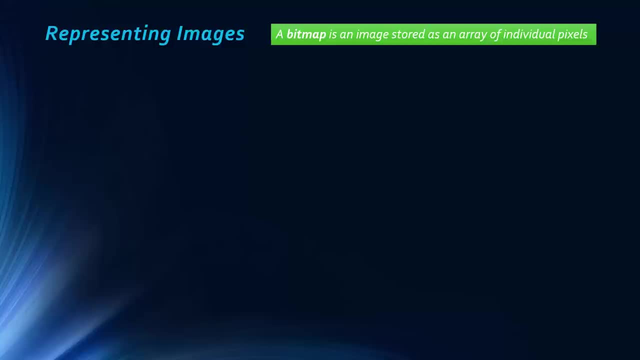 And there's two types of images. we're able to talk about vectors and bitmaps, And vectors aren't on this course, but bitmaps are. So a bitmap is an image stored as an array of individual pixels, So most images are examples of analogue data. 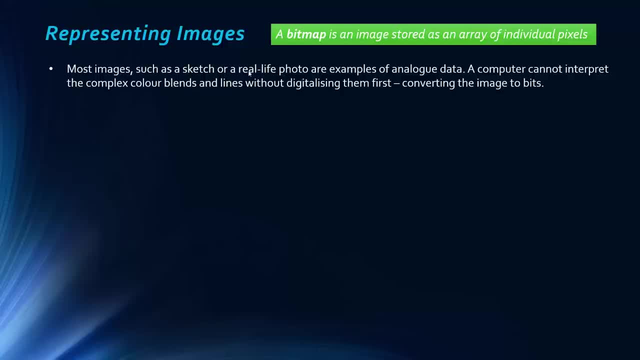 I was just thinking about whether real life photos would really. It's a slight contradiction there, so maybe it's best to talk about in terms of paintings. Essentially, we have this scale of complex colour blends And we have to convert them to binaries. 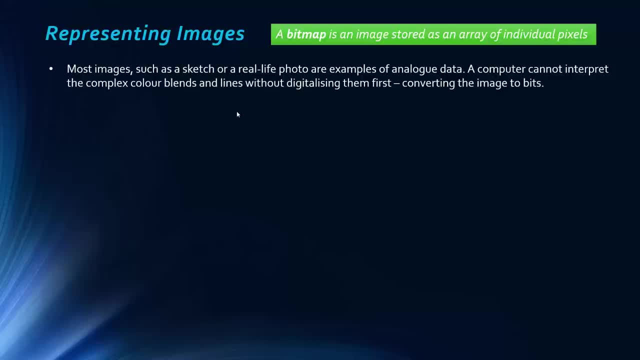 We have to digitalise the analogue data And we're going to talk about analogue and digital a lot more as this video progresses. So a pixel is an individual picture element. It's relatively difficult to define it, but picture element is how pixel is joined together. 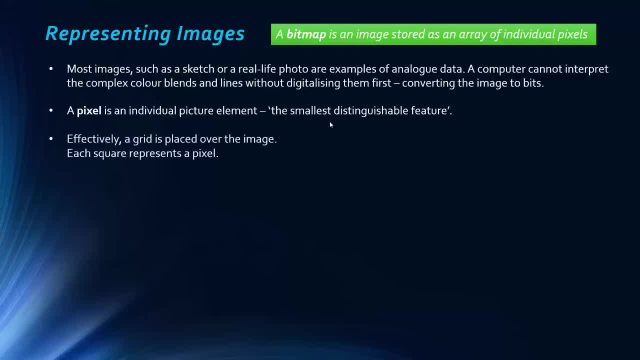 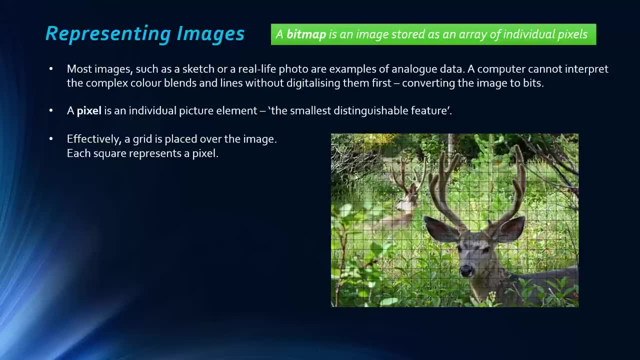 And really it's the smallest distinguishable feature, so kind of like a dot, And so effectively what WAVES has done converted to bits. A grid is placed over the image. Each square, in this case, is representing a pixel. Obviously, this image would look awful. 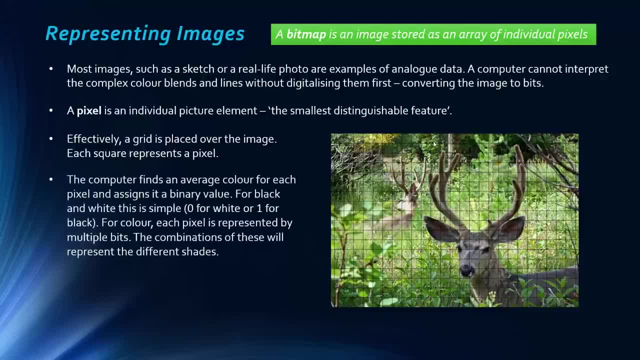 It would be a much smaller grid, Or that's how I like to imagine it. And so the computer finds an average colour for each pixel and assigns it a binary value. So for black and white it's just going to be 0 or 1.. 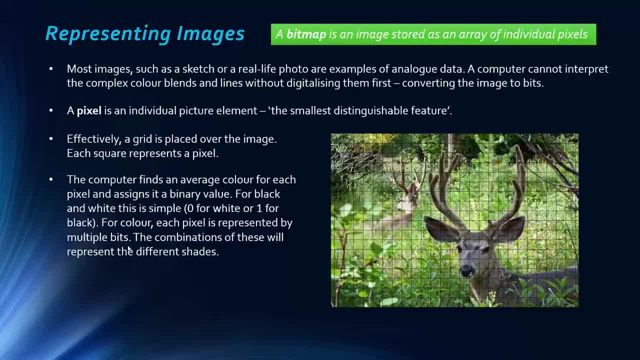 Very simple, But for colour, each pixel is going to be represented by multiple bits. Because you want this colour, you want shades, And so the combinations represent the different shades, And the number of bits allocated to represent each pixel's colour is something called the colour depth. 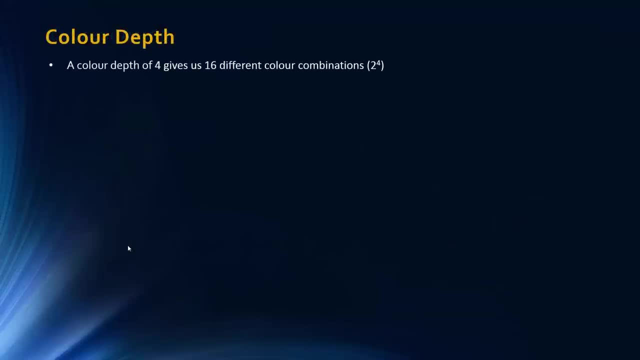 So, if we look at this in more detail, if we had a colour depth of 4 bits, this would give us 16 different colour combinations. So that's 2 to the power of 4. Whereas a colour depth of 24 bits, which might not seem a massive amount, more 6 times. 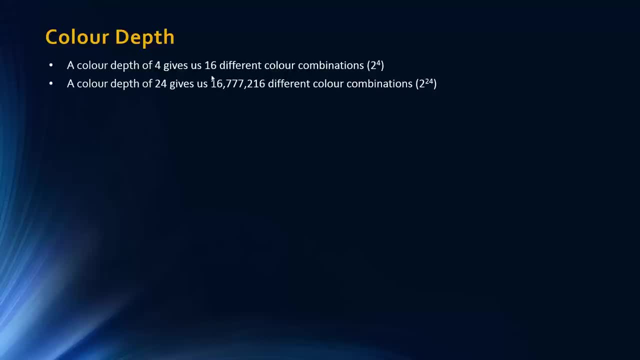 gives us an enormously different massive number compared to 16 different colour combinations. So over, I mean, it's nearly 17 million. That's 2 to the power of 24. And it's just the nature of exponential growth, And so really the number of colours we can represent is constrained. 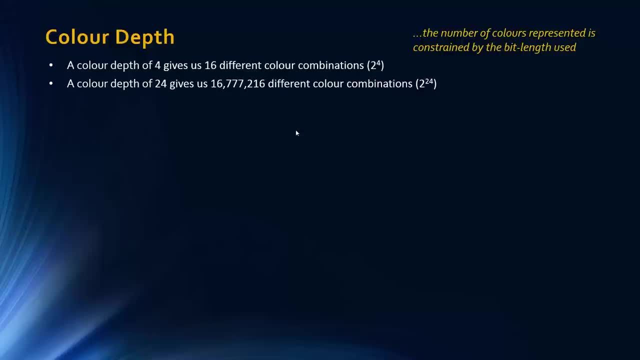 by the bit length used. We only have a set amount of space of memory to store the colours, the colour combinations, And so we are limited by the bit length we use, And the bit length is just how many bits are used to represent something. 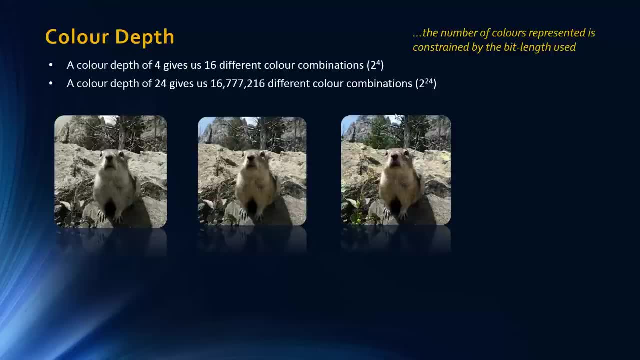 So if we just see this in action of how the colour depth affects the image quality, you can see as we increase the colour depth. it's also called bit depth. so colour depth and bit depth are the same thing. You can see as we're increasing the colour depth. 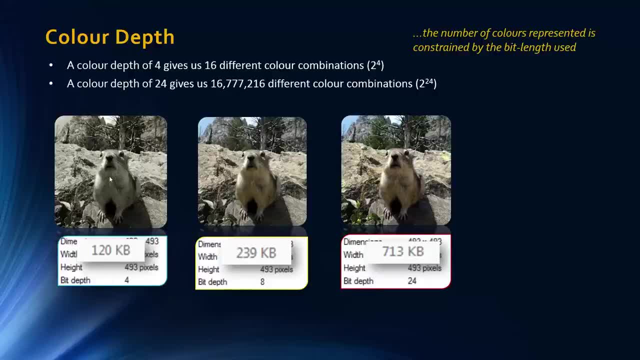 the actual quality of the image gets better. Hopefully you can see this. This is much more vivid. The colours are more natural. So as you increase the colour depth it becomes more and more like the original analogue representation And I guess, by nature, as you increase these number of combinations. 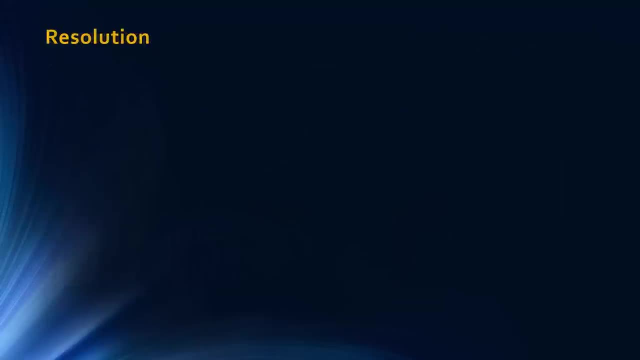 the file size is going to increase too. So the last thing in terms of images we need to look at is its resolution. So the resolution of an image is the detail it holds. So a higher resolution leads to a greater quality image. So we can define resolution in terms of the width multiplied by the height of an image. 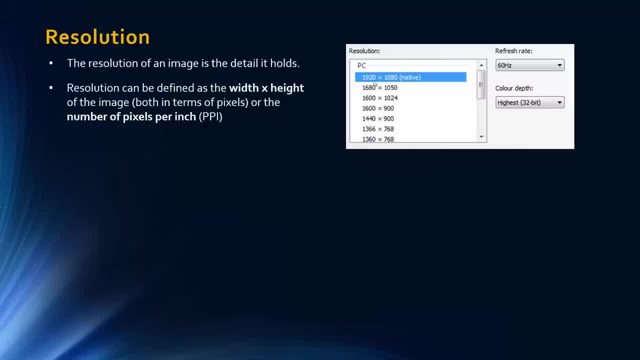 So, like the resolution of a screen is defined like this, Whereas you can also define it in terms of the number of pixels per inch, or dots per inch sometimes. So, when the resolution increases, the grid becomes more detailed, and so you get higher quality. 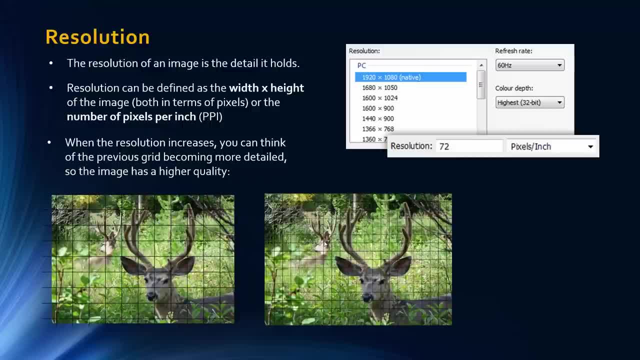 As I mentioned. So you can think of it as the grid getting smaller. That's quite a basic representation. And again, as you increase the resolution, the file size is going to inevitably go up. Okay, I said we're going to keep looking at it. 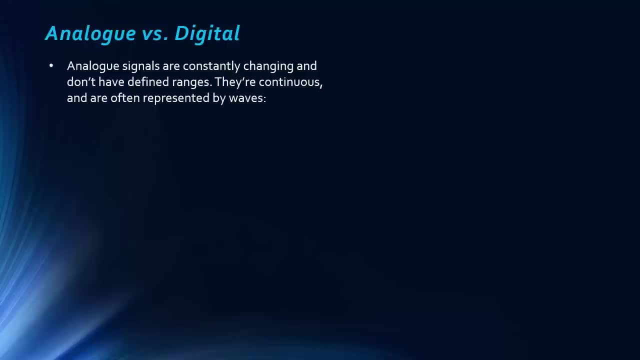 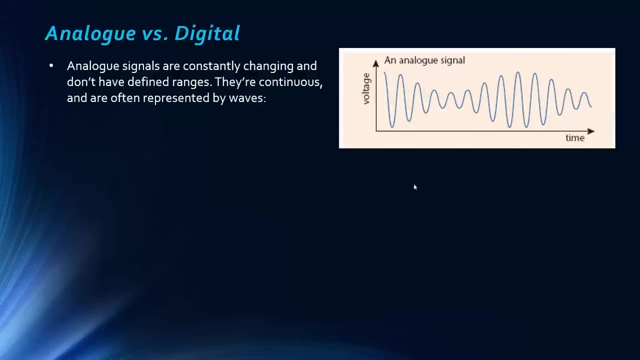 So analogue and digital data. So analogue signals are those that are constantly changing and don't have defined ranges and they're continuous, So there aren't any breaks in between them And so often we represent them with waves, So this would be an analogue signal. 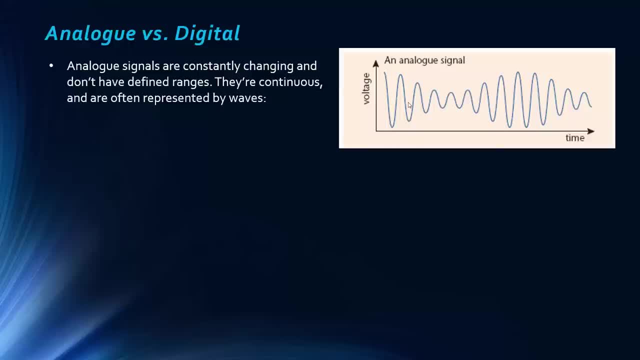 This could be representing sound. So I'm using a microphone now My voice is analogue data because the voice is continuous data And basically pretty much most analogue signals are naturally occurring, And so the voltage on our axis of the microphone I'm using is going to convert the sound waves into analogue electrical data. 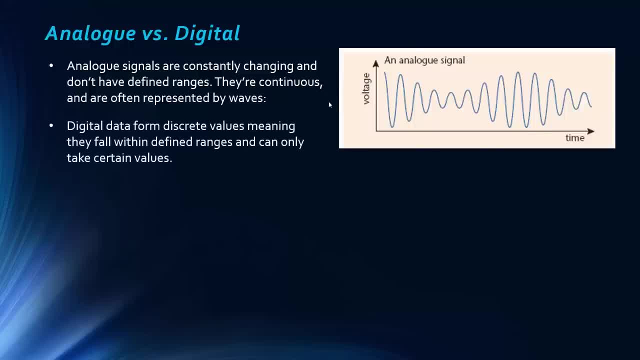 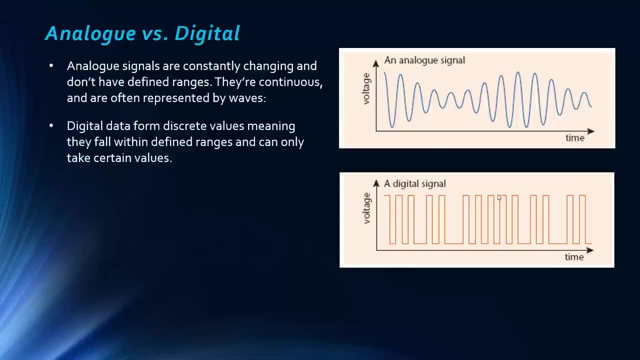 which is represented by the voltage. This contrasts with digital data, which is within discrete values, And this means we only have- we have defined ranges. So this is just zero and one, I guess, for binary system, And it can only take certain values too. 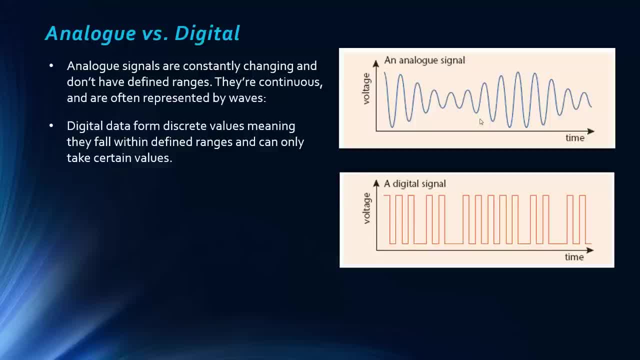 So, whereas analogue data could in theory be any value, digital data is within two set ranges And so the fact for input and output to a computer often analogue. so, speakers, we get sound out from a computer and, like I say, the microphone going in. 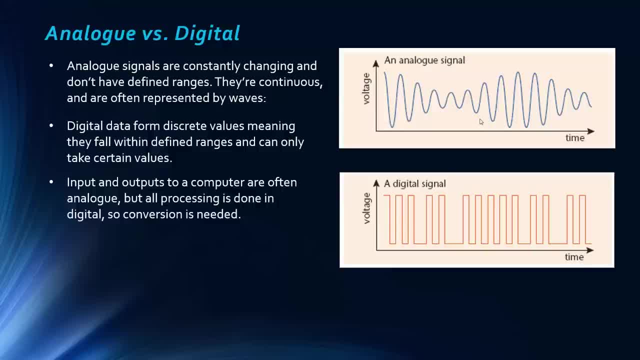 But all processing is done in digital, with binary, So we need to do some conversion, And a device called an analogue to digital converter would perform this task, often shortened to ADC, And the specification mentions three types of analogue data: sound, temperature and light intensity. 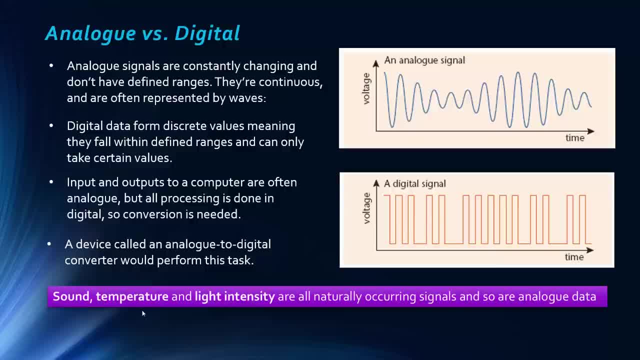 We're going to look at sound. You don't really talk about representing temperature and light intensity because they're not really common inputs to a computer, But if you got asked about temperature or light intensity, we're going to look at sound in a minute. 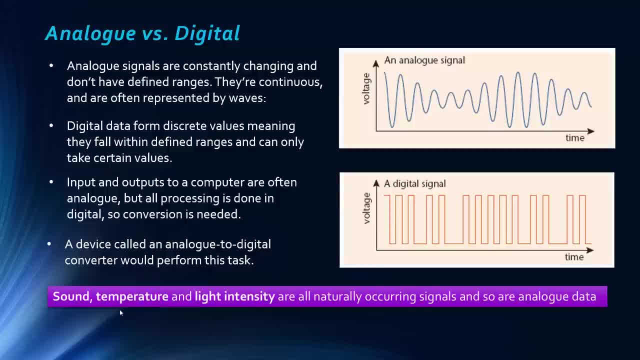 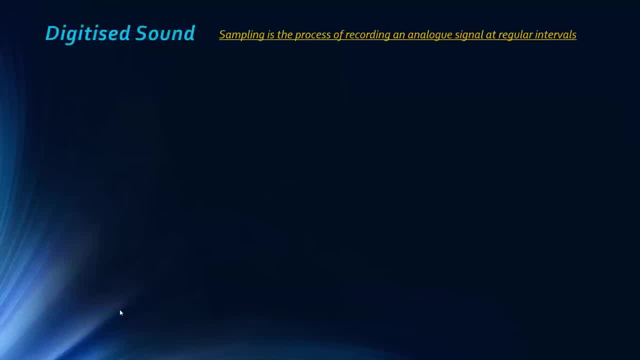 You kind of have to model sound and just replace what you're talking about of sound with temperature or light intensity. It's a very similar process. So first of all we're going to look at sampling, And sampling is a process of recording an analogue signal. 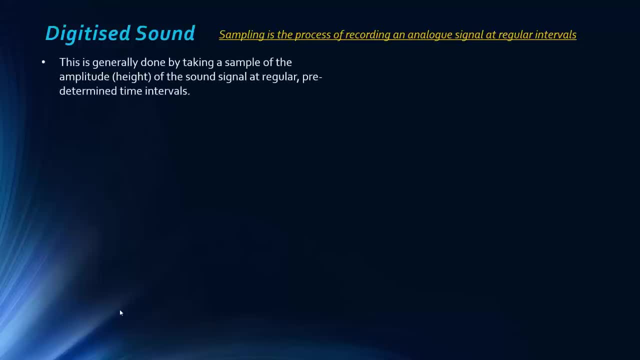 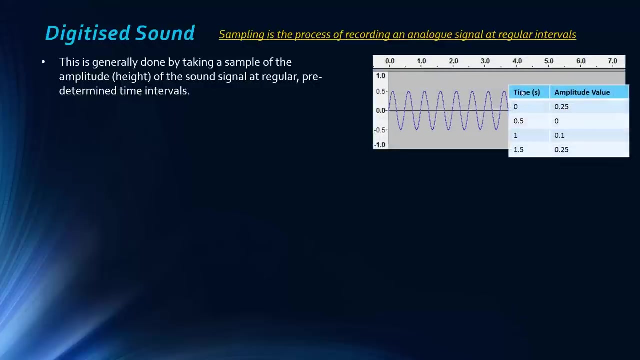 at regular intervals And this essentially means it's converted to digital. So it's done by taking a sample of the height or the amplitude of a signal at regular, predetermined intervals. So, to be honest, I did this over a year ago. this little bit for a previous course I covered. 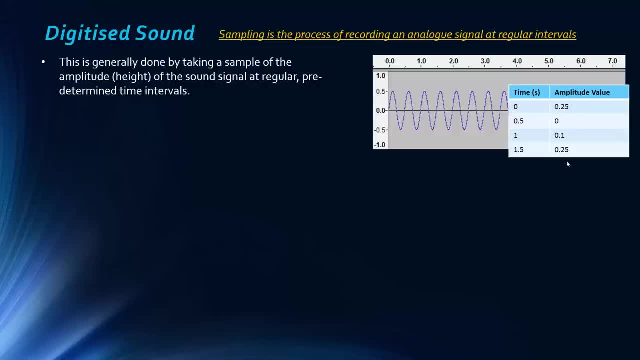 I don't really know what I'm doing here because I'm not convinced by the values. I might have just made it up. If you can see what I'm doing, I'm recording the amplitude value at different time intervals, So the set interval is 0.5 seconds here. 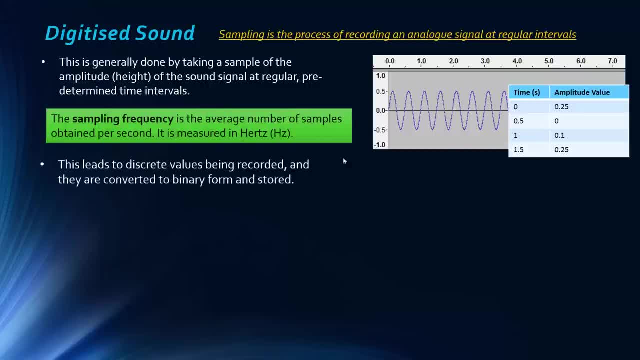 And I'm recording the time interval And then this will be stored as a binary value And the sampling frequency is a term you need to know And that is the average number of samples obtained per second. So the average number of samples recorded per second: 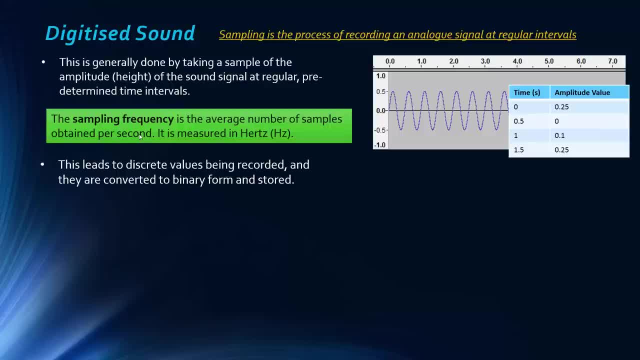 And the unit we give it is hertz. Also, it might be written as samples per second, because hertz is 1 over s, And so the more frequent you sample it, so a higher sampling frequency, the more true the representation is to the original analogue signal. 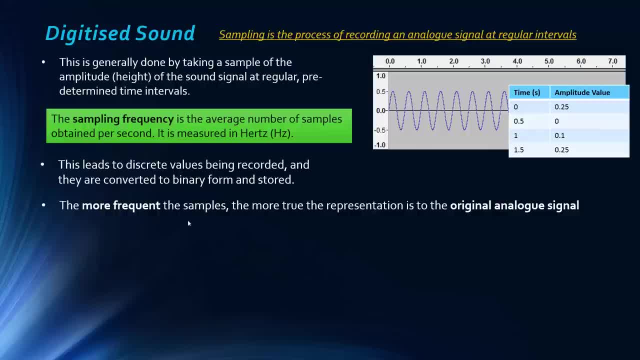 So this is a limitation of sampling. Whereas analogue there's a value at every single point, you're only taking a sample at certain points, So you're going to be missing some of the actual original analogue signal. But the more you do it, the more true it is to the original signal. 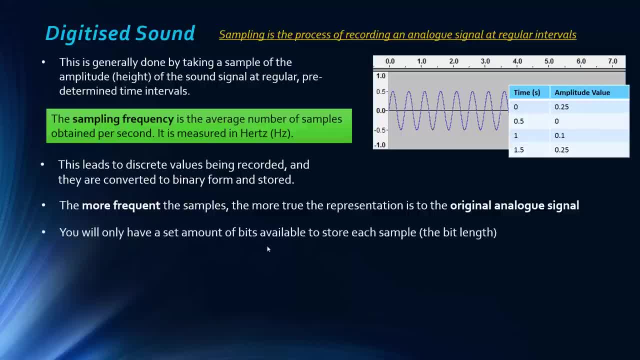 And so because you only have a set amount of bytes- sorry, a set amount of bits available to store each sample- and this is again the bit length- you're limited in how many values you can record. So if we only had 4 bits to store each sample, 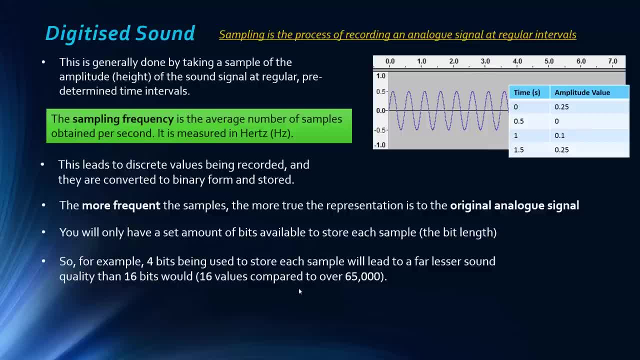 so each value we're going to lead to our sound quality was not as good as if we used 16 bits, And so this would be 16 values, which is 2 to the power of 4, compared to over 65,000,, which is 2 to the power of 16.. 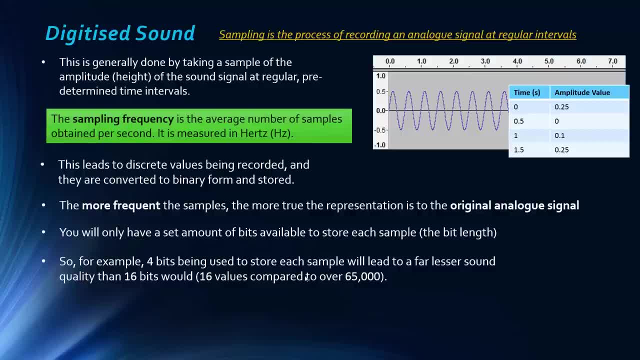 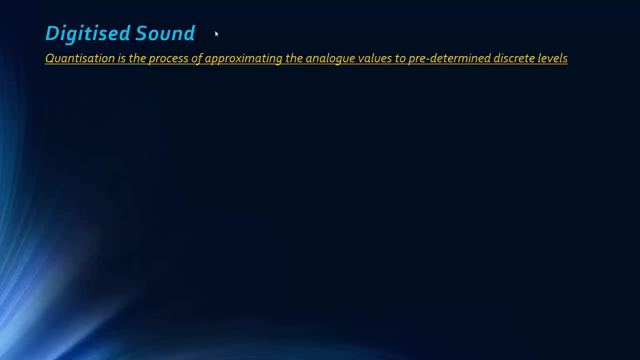 And so again, we're constrained. The quality is constrained to how many bits we're using to store each value and how many times we're sampling it Another way. or we need to look at something called quantization. This is a process of approximating the analogue values. 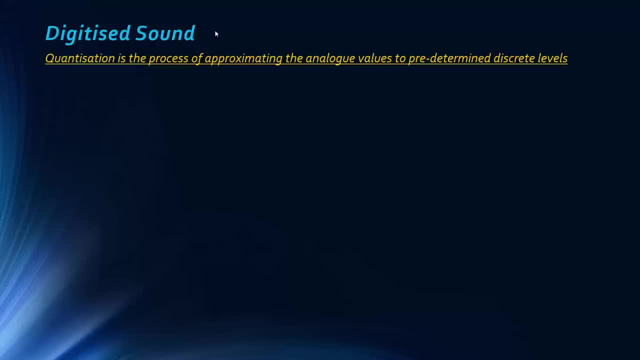 to predetermine discrete levels, And so this is actually something I had to look up. I've used this kind of similar process in maths before- briefly, but this is obviously in terms of sound and signals, And so I'm not a sound engineer. 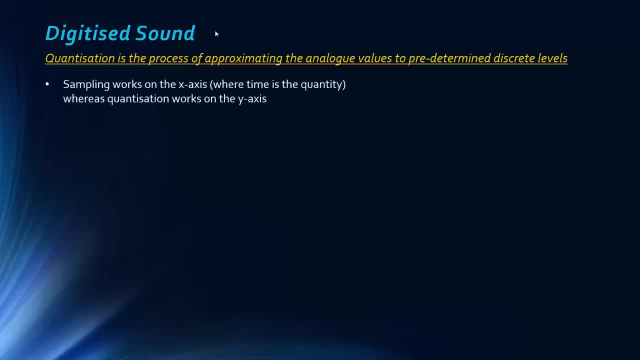 so I've tried to look it up, but it's not massively. I found it quite difficult to understand fully, but I did my best to try and explain what I think I understood. So sampling is something that works on the x-axis. We're working on the x-axis where time is a quantity. 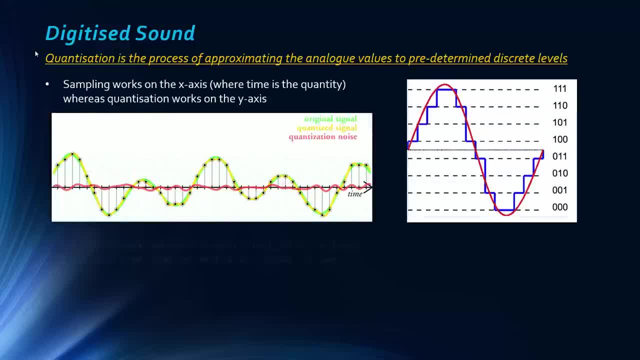 Whereas quantization is working on the y-axis. So really what we're doing is we're mapping the original analogue signal to the closest digital value we've got set. And so you can see here- and I've taken this from Wikipedia- the original signal is in green. 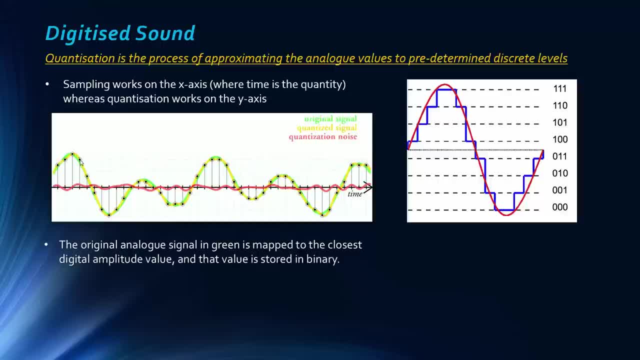 and we've got these set levels to store it at. So we're trying to make it into a discrete set of data And so we're basically just approximating it by mapping it towards the closest level available. So we are losing some of the actual original signal. 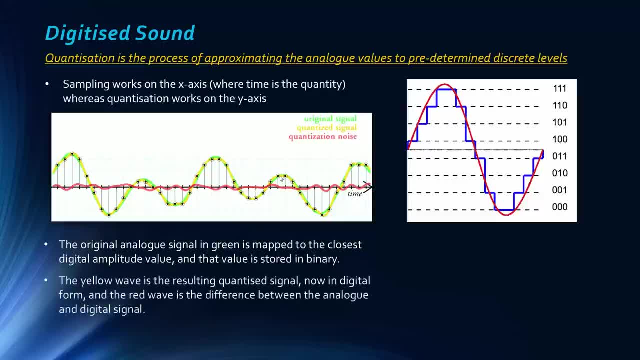 You can see in red we've got the actual difference between the original and the quantized signal. So the quantized signal is the digital signal. So it's not perfect and we are going to lose some of the actual true sound, but it's just another way of digitizing the sound. 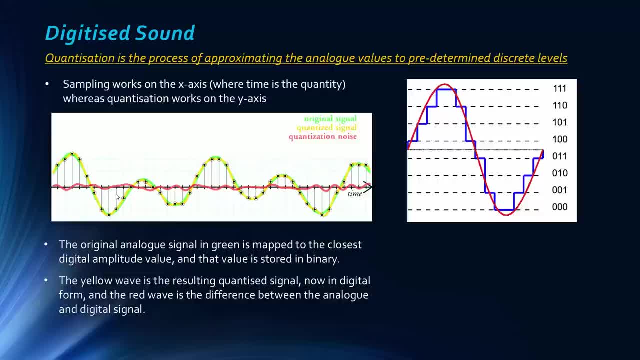 And I think sampling and quantization are used together. but, like I said, I'm not a sound engineer, so I don't totally understand the actual process. but we can look at it from a computer science perspective And we can talk about that if we are only using three bits. 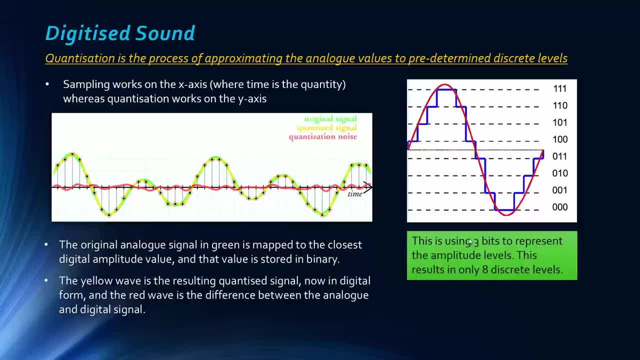 to represent the amplitude levels. we're only going to get eight discrete levels possible. So this is again from Wikipedia. We see we've got three bits used to represent each level and this means we've only got eight actual possibilities, because two to the power of three is eight. 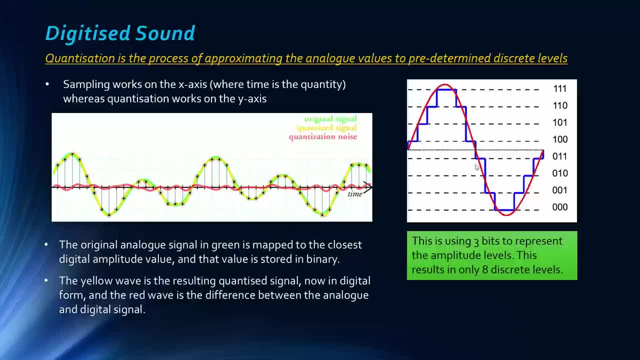 And so it means we get quite a jagged sound here. It's not nearly accurate, So this is relatively smooth or very smooth, So this is obviously pretty good, whereas this is using not many bits to represent each amplitude level, so we get quite a jagged sound representation. 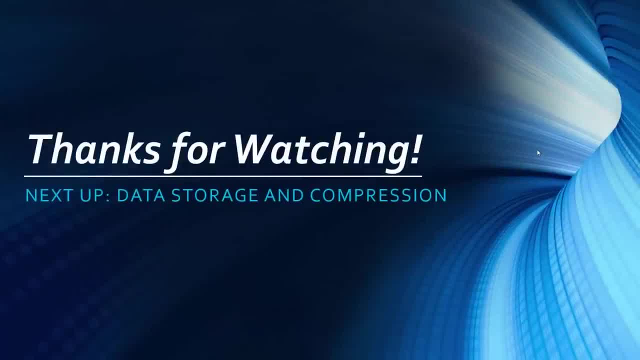 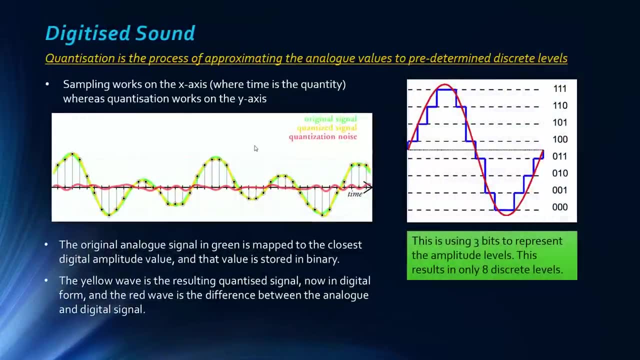 So that's it for this topic. Quite a difficult one, I think The sound is slightly difficult. Like I say, if you do get asked about this in terms of light intensity or temperature, just try and model it on what we've looked at with sound. 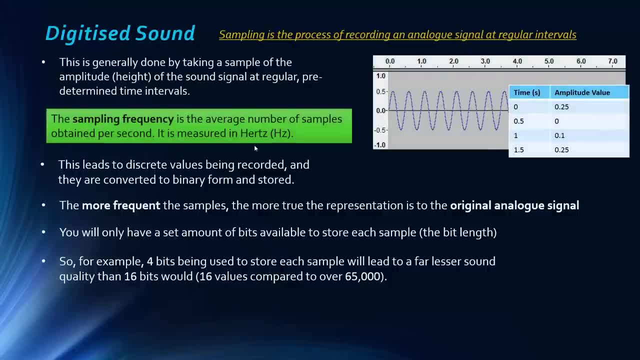 It's basically the same process. If you get a choice, I'll talk about sampling, because it's slightly more intuitive And you really just got to talk about. so, talking about temperature, you've got to take about the input, you've got to record the amplitude at set samples.